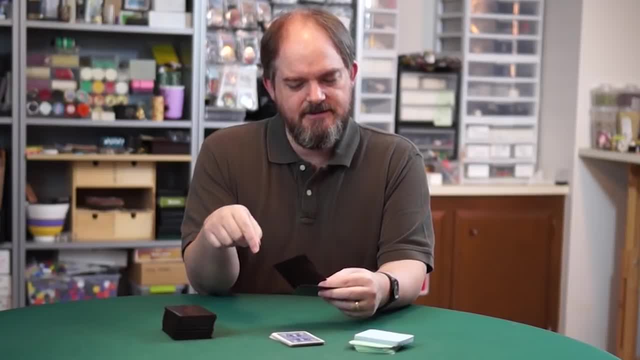 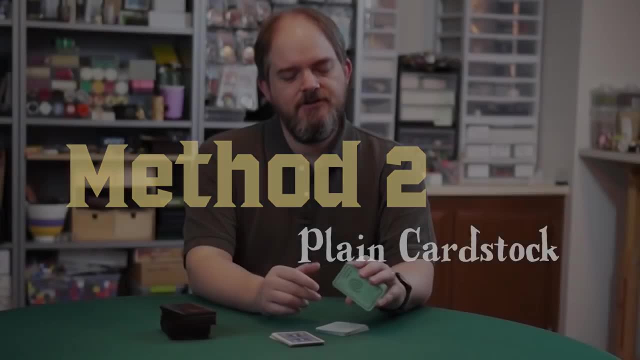 cutter for it, and the reason I say it's cheap is that the cards and the sleeves are reusable, so all you're really blowing through is the white paper that you printed it on. Method 2 is just to print the cards on card stock like this. This is a little more labor intensive. 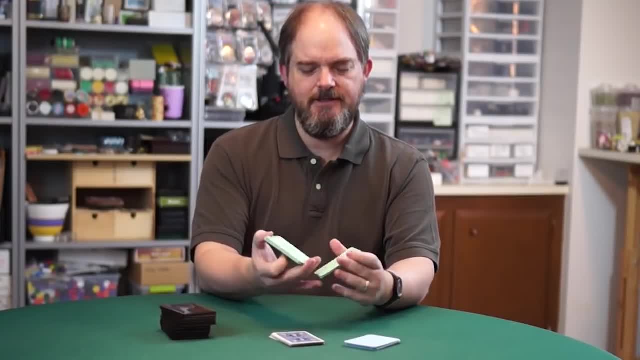 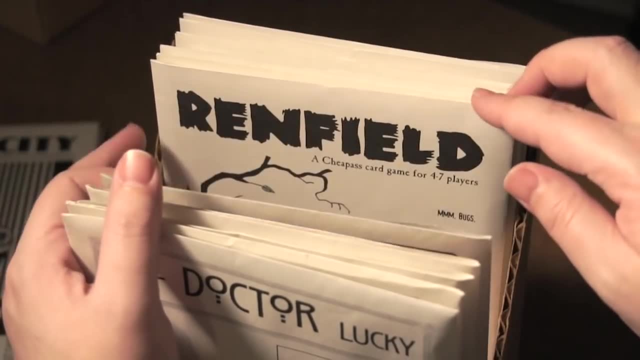 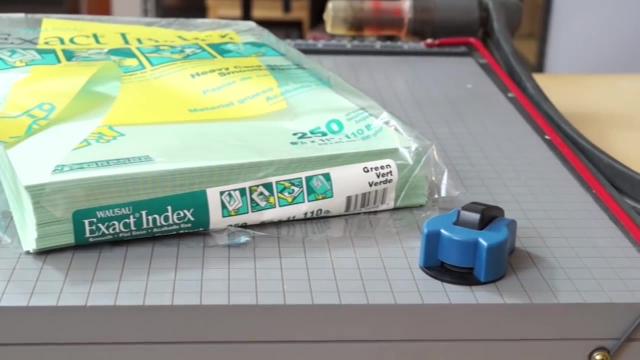 as you'll see, but it's good for some applications, especially if you want to duplicate the look and feel of the old-fashioned cheap-ass games which were made exactly like this. For this you just need a good card stock, like 110 pound index, and a good paper cutter. Optionally, you can also use a. 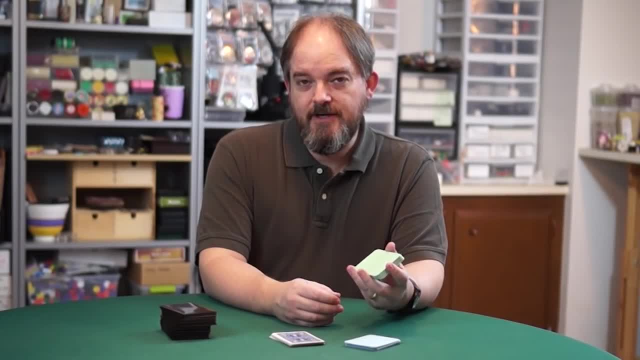 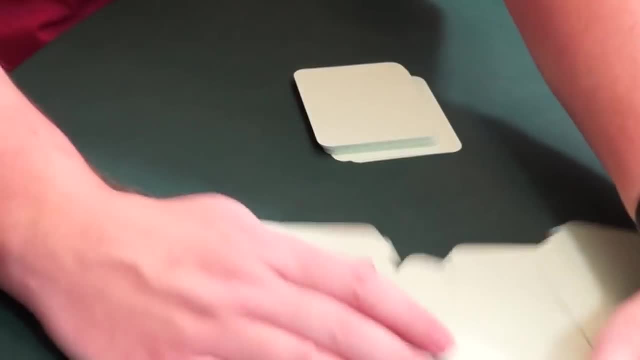 corner rounder. This method works best for black and white cards, which I can do on a laser printer, partially because I'm printing right on the surface and this is going to get a lot of wear. Inkjet will get wet and rub off and laser toner will stay a little better. So start by printing. 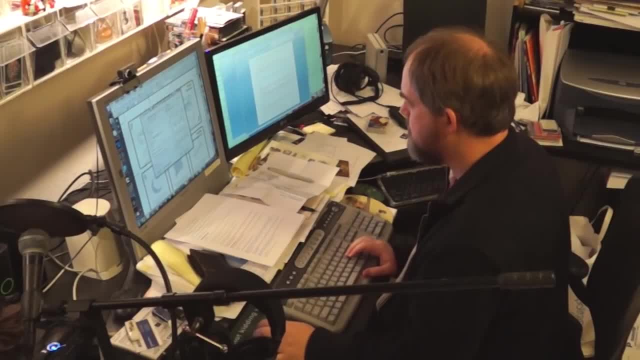 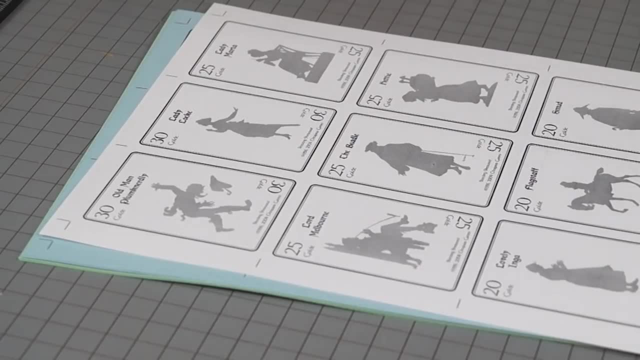 the cards on the card stock and print a guide sheet as well. that's going to help you do the cutting. If the card file doesn't have a guide sheet or if you can't just make one, then print an extra copy of page one and use that to lay out your cuts, Take your guide sheet and extend those. 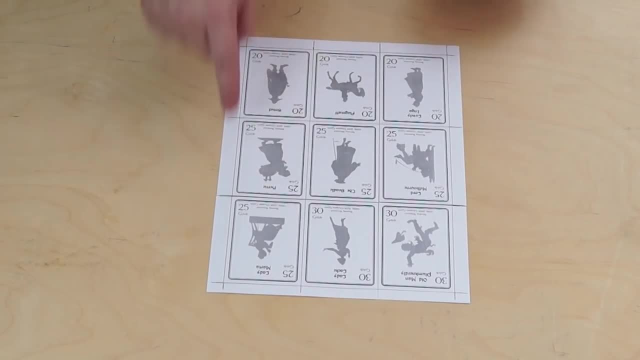 crop lines all the way to the edge of the page. We're not going to trim around the outside. first We're going to make two bust cuts down the middle of this page. We're going to separate into four sections and then we're going to clean up the edges. 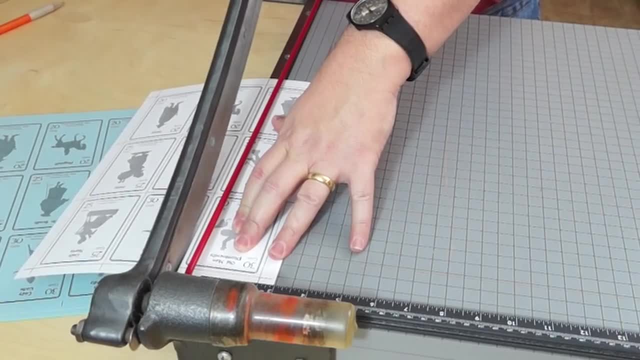 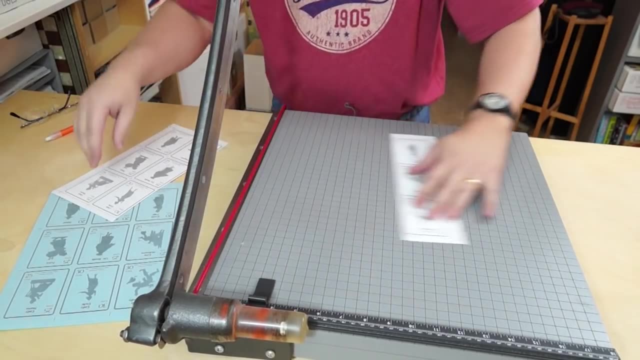 The reason you do that is, as you cut the sheet you're going to have some creep and you want to minimize that by starting a good clean cut right in the middle. Use the cutter's backstop on this so you can make the same bust cut on every sheet After you've done one direction. 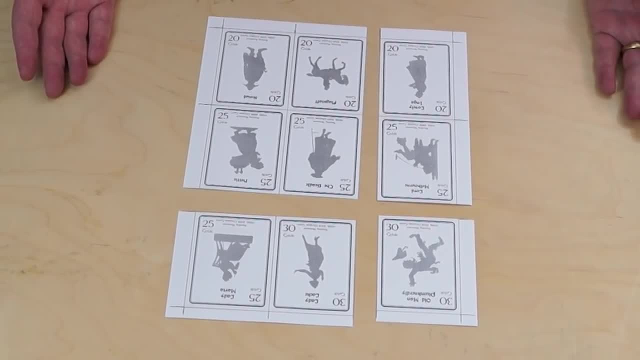 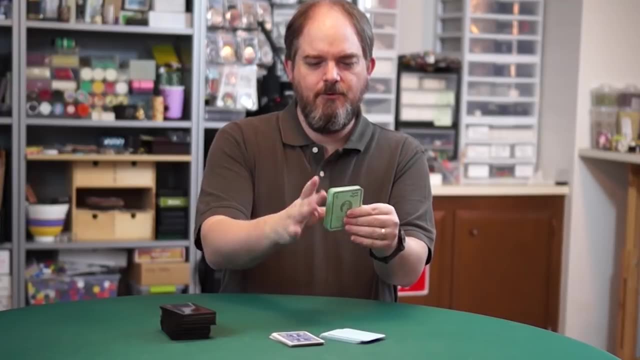 you're going to cut the other direction. You're going to wind up with four quadrants of this page, each with two rough edges. Because you shuffle these cards end to end, the height is more important than the width, So the width is the first cut you're going to make and you're going to save the. 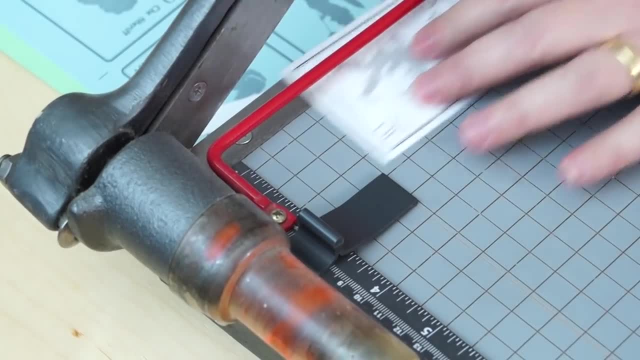 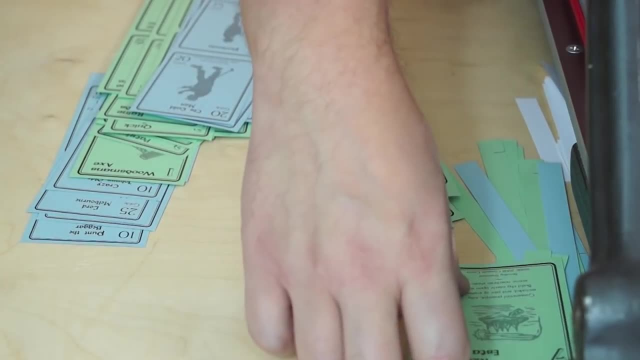 height cut. for the very last cut, Use your guide sheet to set a depth for the width cut and then you lock that setting in for the entire deck. You trim all the cards rough edges off until you just have strips of one or two cards with just one rough edge left. Then you use the same method to mark. 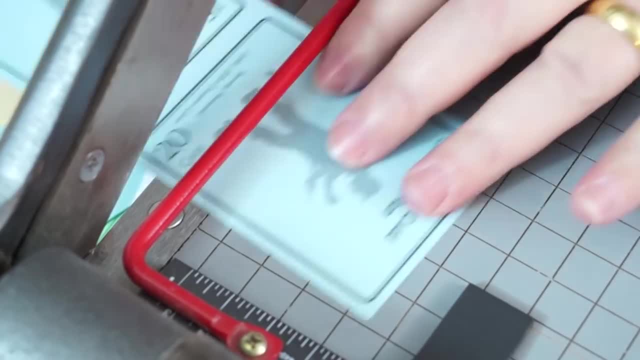 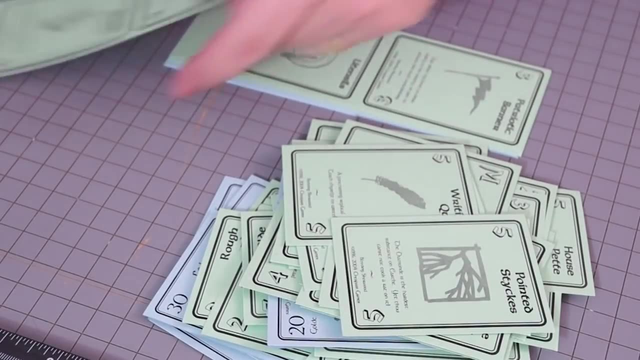 the height of these cards and trim them all down. In this step, you do not care about hitting the crop lines perfectly. You are probably going to miss them. It's more important that all the cards be the same height. That's why cards have margins Now. this is an optional step, but your cards will. probably shuffle a little better if you round the corner. You're going to want to make sure that you make sure that you're making the right cut for the entire deck. You're going to want to make sure that you're making the right cut for the entire deck. You're going to want to make the right cut for the entire deck. 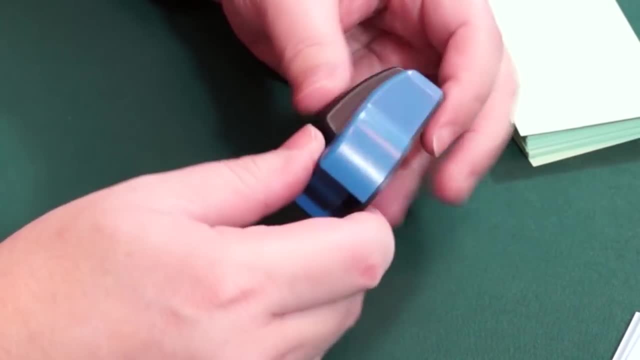 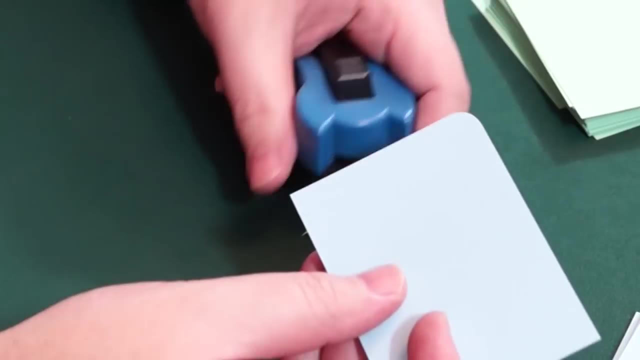 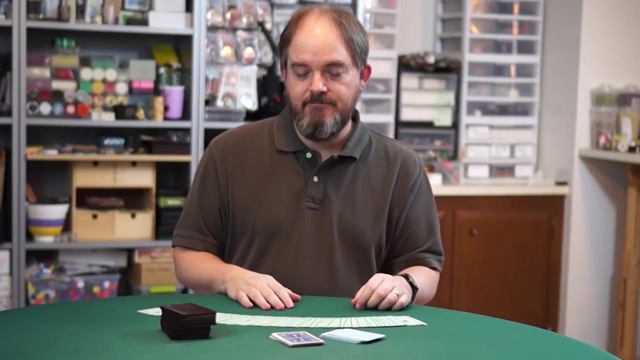 Get a corner rounding tool like this. You can get it from a scrapbooking store and painstakingly clip every corner. These cards can be a lot of work, but they're worth the effort. They're nice and thin, portable, shufflable and fairly cheap. 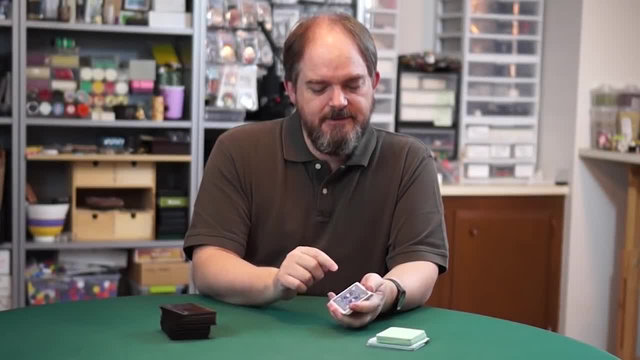 Method three is to stick labels on playing cards. I use playing cards specifically for this and cards that have a linen finish, because that linen finish keeps them from sticking together and makes them easier to shuffle. You want to make sure that the cards don't stick to each other when you're. 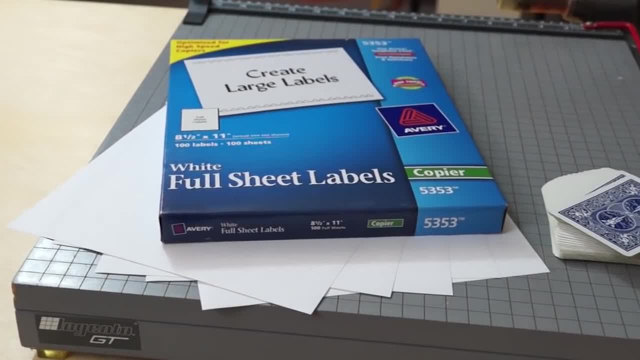 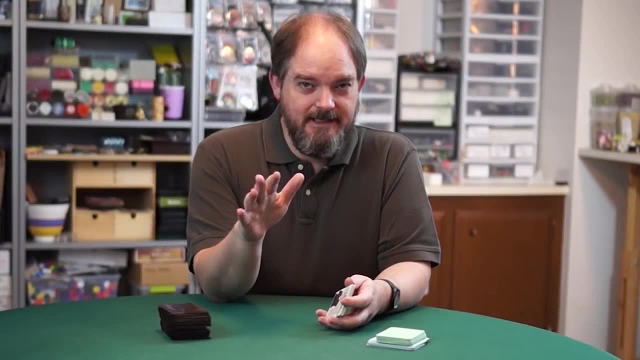 making a shuffle. For this you're going to need full sheet labels, some junk playing cards and your paper cutter. Use full sheet labels for this, not die cut labels. There aren't any labels that are cut to exactly the right size for playing cards, and even if there were, you would have real trouble. 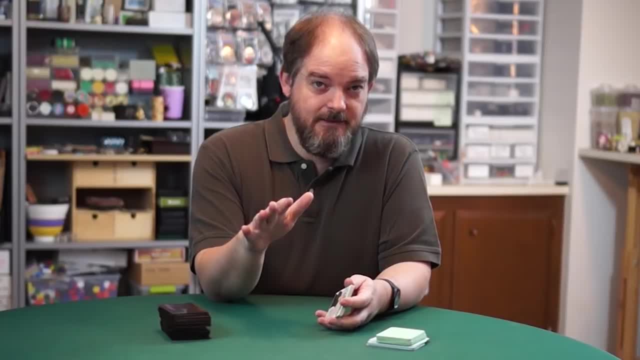 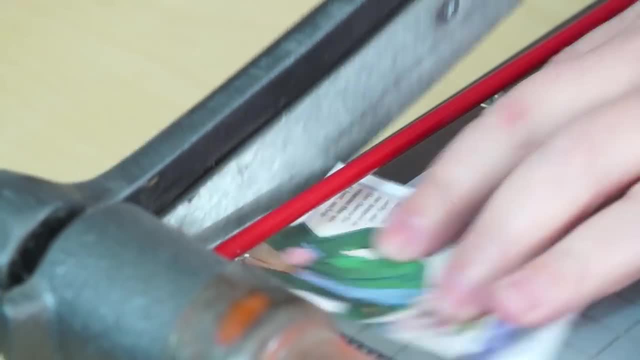 lining them up. You print on a full sheet of labels and then you can chop them up exactly where you need to. For this technique, print your card art at 95 percent. You want it to be a little smaller than what you're sticking it to. You can just eyeball your cutting on this. The cuts don't. 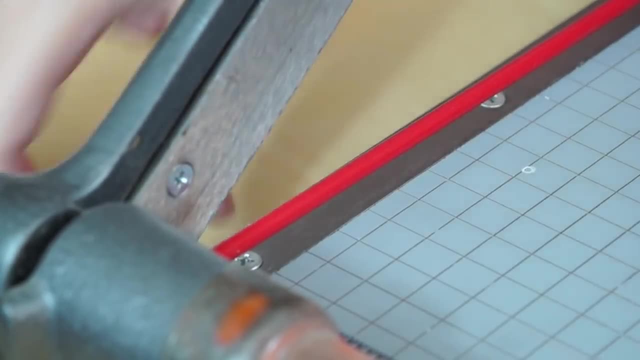 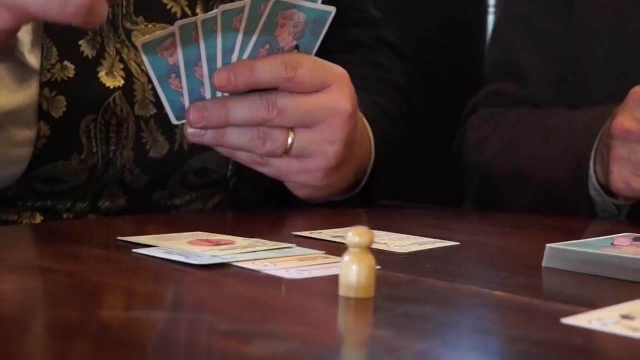 have to be precise. they just have to be small enough to fit on the card. Now stick your labels to the card. I don't typically label the backs of these cards because that screws up the finish and makes them hard to shuffle. It makes the deck really thick. I only sticker the backs if it's for show. so if I 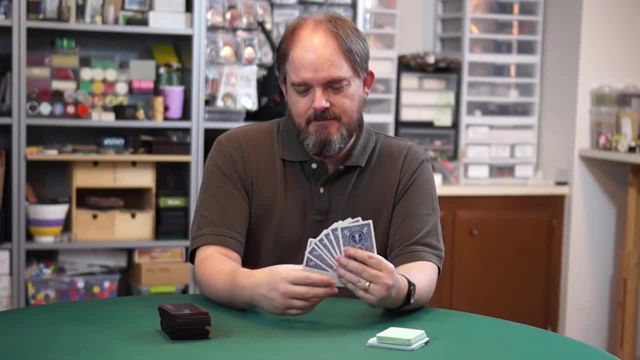 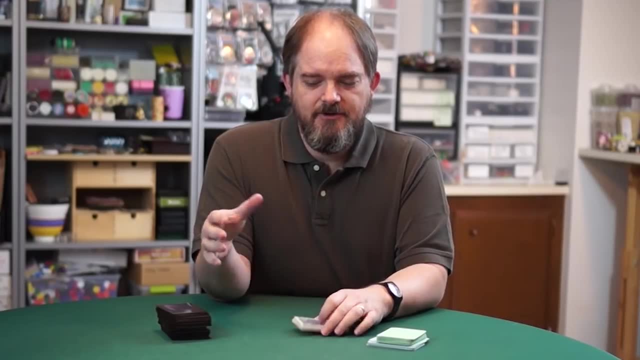 was making a video and I wanted to pretend this was a real copy of the game. I'd sticker the backs. Otherwise, they're much better just using the original cards. And that's method three. There's lots of other techniques for making cards. You can hybridize these techniques or come up with your own. 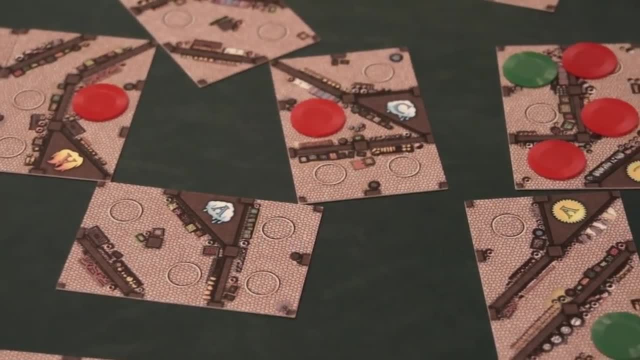 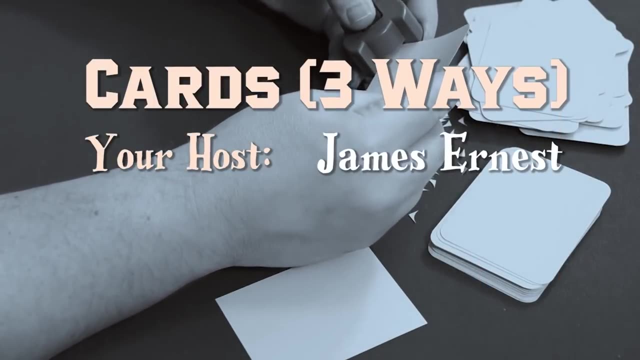 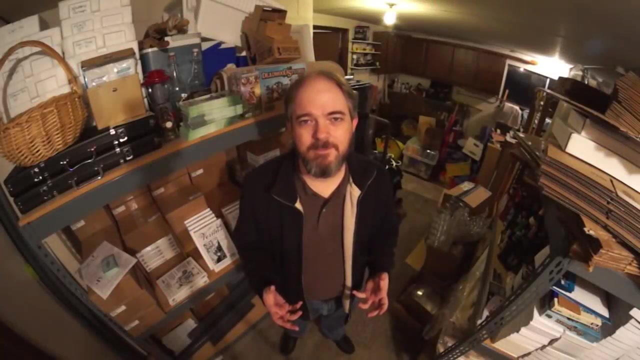 You should also check out my other video on how to make tile cards, for when you're making a game that you actually build the board out of the tiles. Now pick your favorite and go make some cards. Cheapass games come in three varieties: Deluxe, classic and free. Our deluxe games are lavishly.